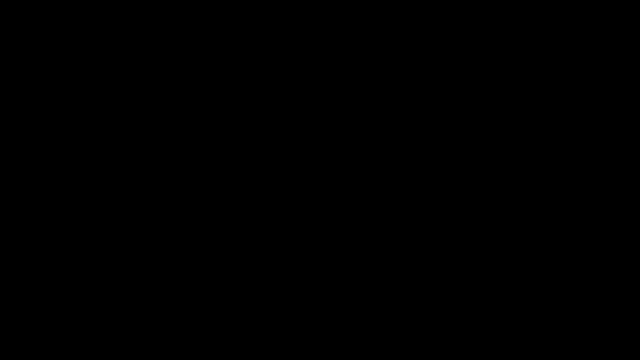 In this video, I want to focus on indirect proofs. So let's start with an example. Let's say: if we have two triangles, Let's call the first one triangle ABC And the second one we're going to call it DEF. Now let's say that we're given the following statements: 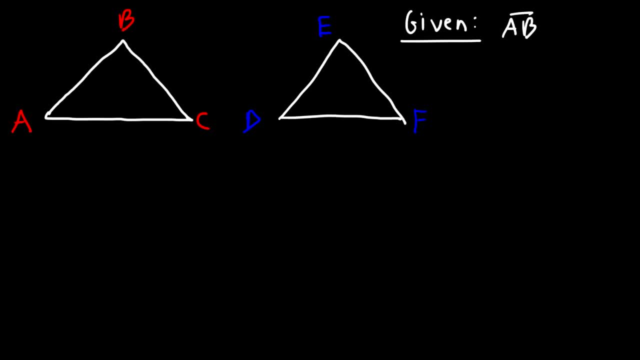 Let's say that AB is congruent to DE, So that's the first given. And let's say that BC is congruent to EF, And let's say AC is not congruent to DF. Your task is to prove this statement, Prove that angle B is not congruent to angle E. So go ahead and try this problem. So let's prove it with two-column proof. So we're going to have statements And we're going to have some reasons. Hopefully I can fit it in in this one page. 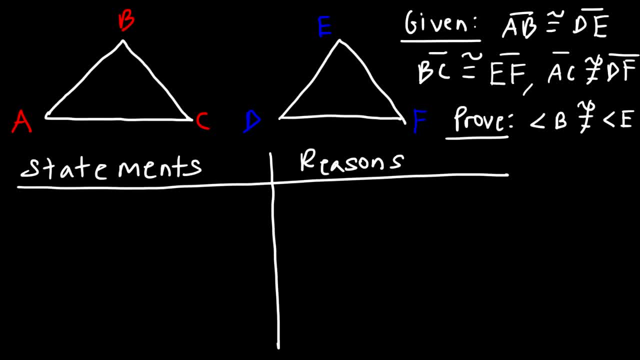 Now how should we begin? The first statement that you should make should be a negation of the conclusion or a negation of the statement you're trying to prove. So we're trying to prove that angle B is not congruent to angle E. Therefore, we're going to make the statement that angle B is congruent to angle E, And so the reason it's an assumption. 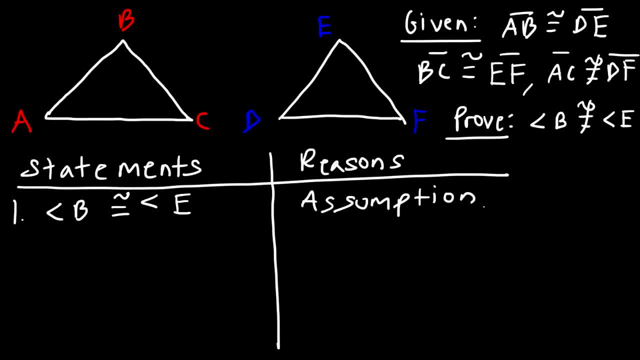 We're going to assume that this is true. Okay, In our attempts to prove this, That it's false, Now the second statement that we're going to make Is that AB is congruent to DE And that was given to us. 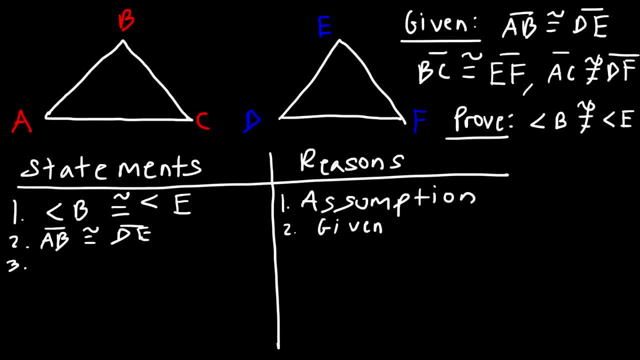 So let's write: given Now number three, Let's put a mark. So AB is congruent to DE, And also we're assuming that angle B is congruent To angle E. So as we write these statements, We should also make the marks on the figures. 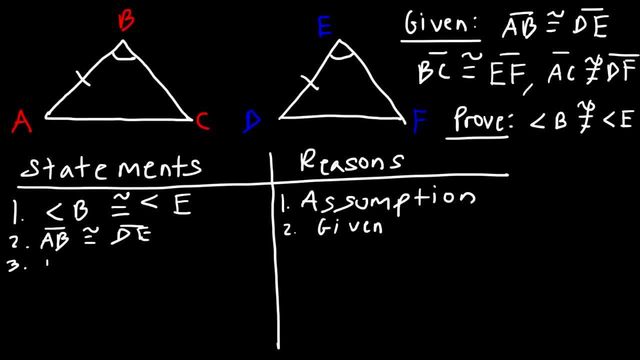 Now the third statement Is that BC Is congruent To EF, So that's also given. Now the fourth statement is this one, That is AC. AC Is not congruent To DF, And so that's given as well. 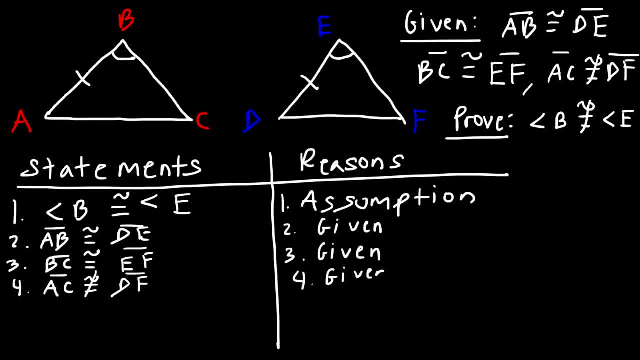 And we said that BC is congruent to EF. So these two sides are the same. Now notice that we can prove That this triangle Is congruent to that triangle, Based on the side angle, Side postulate. So we're going to make this statement. 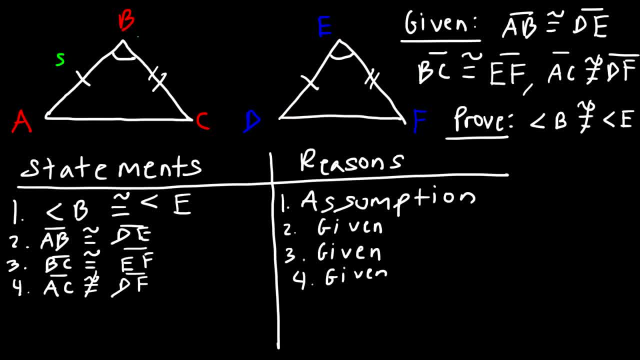 That this triangle is congruent to that triangle Based on the side angle Side postulate. So we're going to make this statement: That triangle ABC Is congruent To triangle DEF, And so The reason for this. 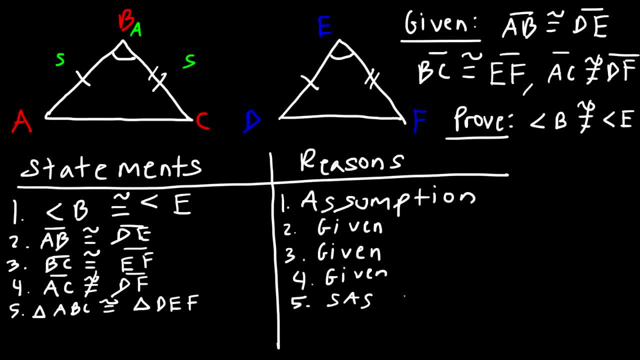 Is side angle, side The SAS postulate, And for this one We've used statements two. AB is congruent to DE And for the angle That was statement one, Angle B is congruent to DE. That was congruent to angle E. 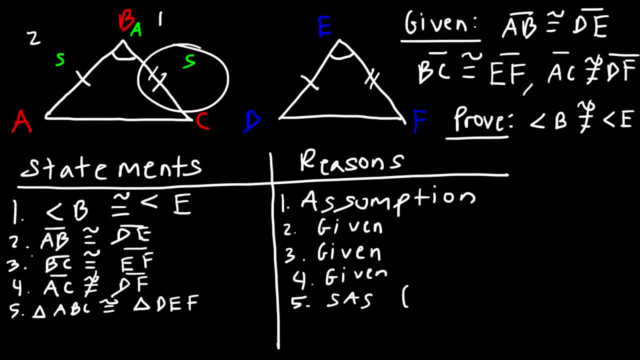 And For this one, BC is congruent to EF. That was based on statement three, So it's side angle side, Based on statements Two, one and three, If you want to go in order From left to right. So now that we've proven, 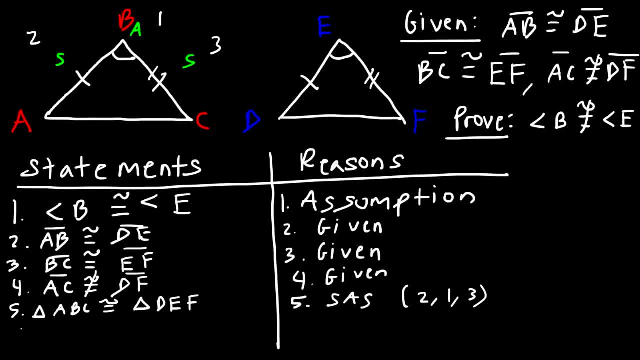 That these two triangles are congruent. What should we do next? Statement six: So now We can focus on The statement that was false. If these two triangles Are congruent, Then we can say that AC Should be congruent. 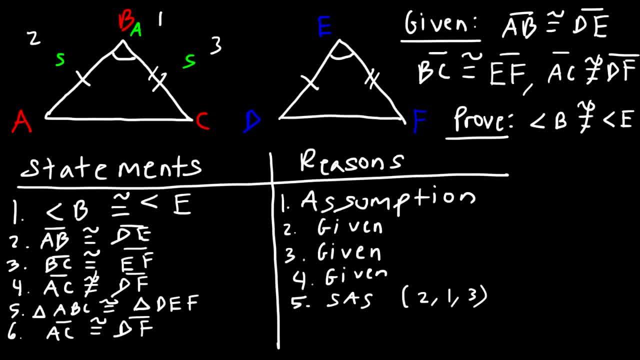 To DF Because the two triangles are congruent. If you have two congruent triangles, Every part of those two triangles should be congruent. That means AC Should equal DF According to CPCTC, Corresponding parts Of congruent triangles. 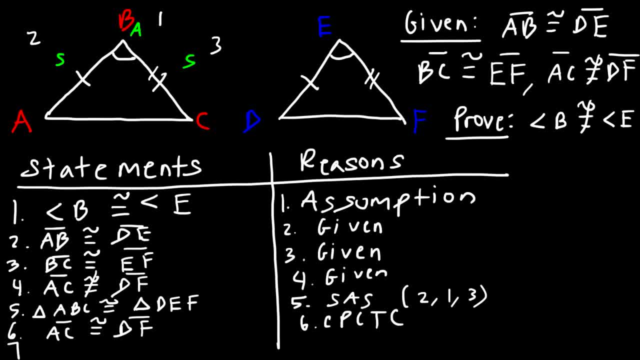 Are congruent. So now let's move on to statement seven. Notice that statement six And statement four, These statements Contradict each other. Statement four is saying that AC Is not congruent to DF, But statement six is saying that AC. 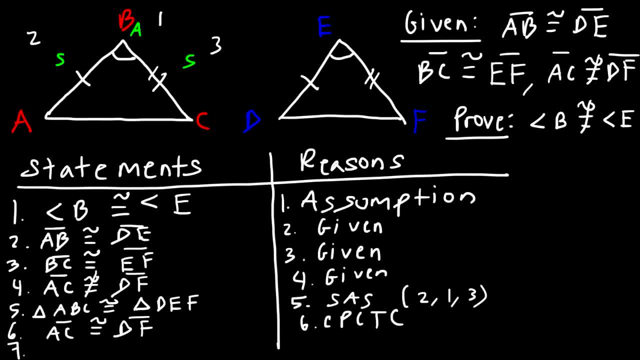 Is congruent to DF, So there's a problem. So, because those two statements Contradict each other, The assumption was false. Therefore, angle B Is not congruent To angle E. So for statement seven Or for reason seven, 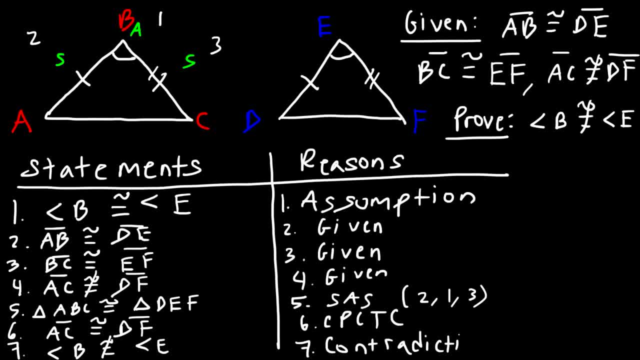 We can say: this is due to a contradiction Of statements Four and six, And so that's it. That's how you can Use an indirect proof To prove that angle B Is not congruent to angle E, The key. 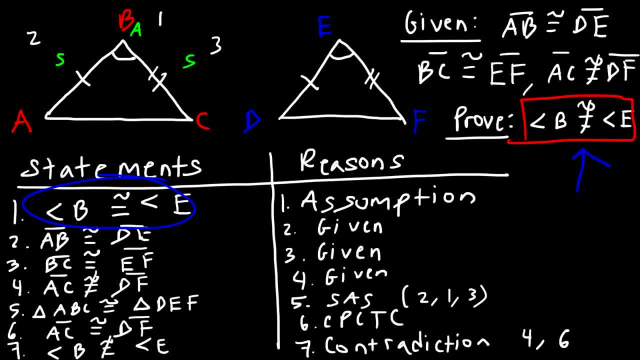 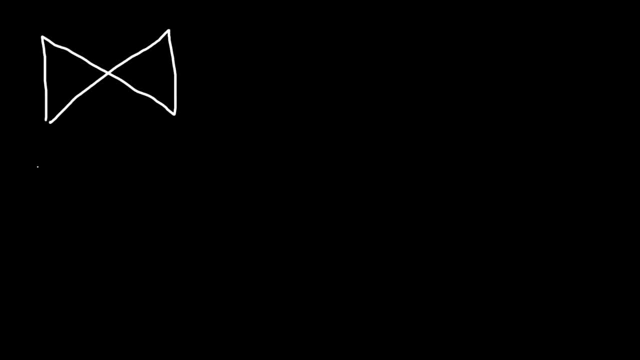 Is to start with an assumption, And that assumption is the negation Of what you're trying to prove. Let's try another problem. So let's say this is A, B, C, D and E, And so in this problem, 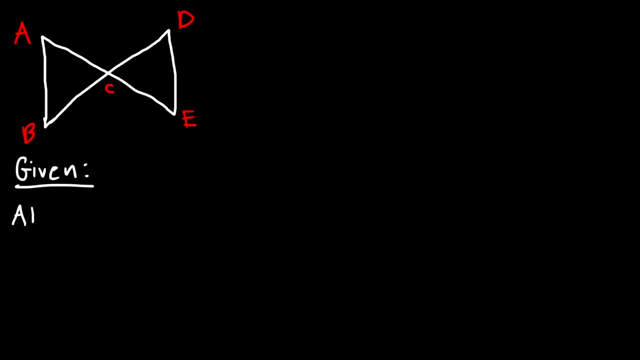 So we're given that A- B Is congruent To E- D And also B C Is congruent To D- C, And we're also told that A- C Is not congruent To E C. 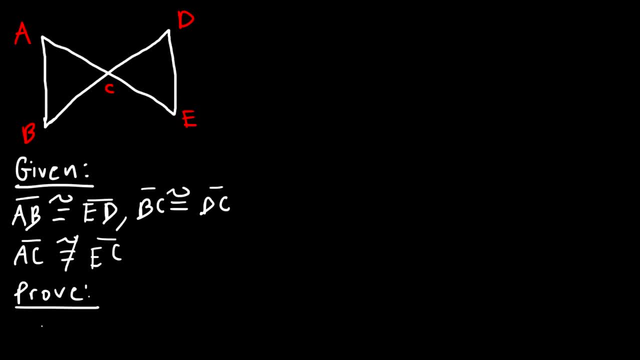 Your task is to prove That angle B Is not congruent To angle D. So, based on the last example, Go ahead and try this problem. It's very similar to last example, so This should be a good practice Problem for you to work on. 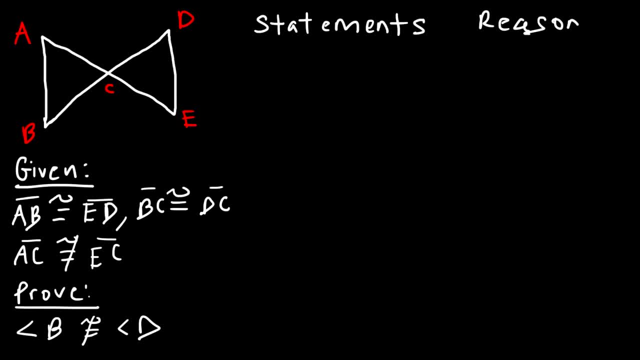 So use a two column proof To prove that Angle B does not equal Angle D. So So, once again, We are going to assume the negation Of our conclusion. So in the first statement We're going to say that angle B 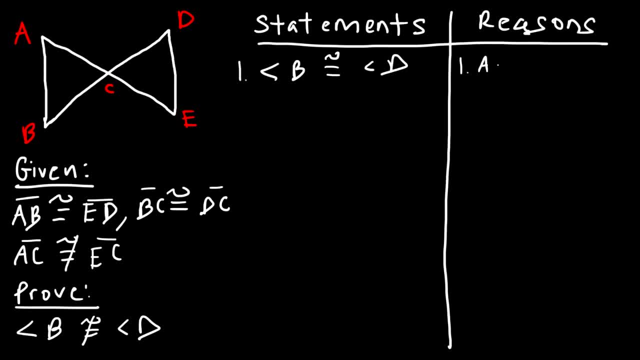 Is congruent To angle D, And so the reason We're going to assume, We're going to make an assumption, And so let's mark that on the graph. So angle B Is congruent to angle D. Now number two. 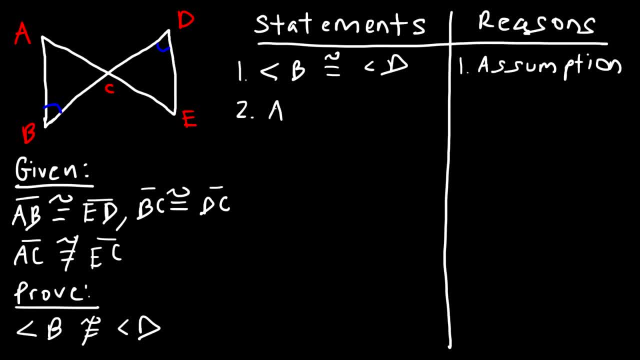 Here we have our first Statement, So we can say that AB Is congruent To ED And so that's given And we can mark that as well. So those two sides are congruent. Now statement three is the next given. 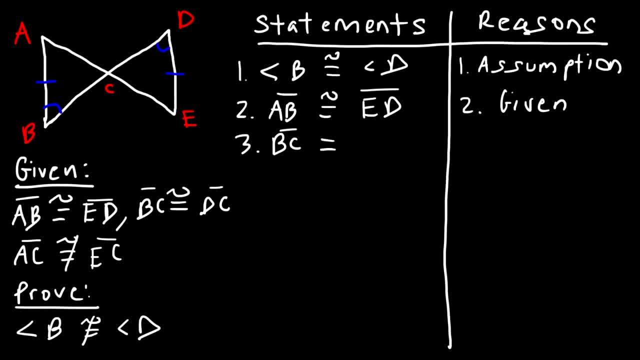 We can say that BC Is congruent To DC. So here's BC And here's DC. And then here's the last given statement. So let's rewrite that AC is not congruent To EC. Now I'm not going to mark anything on. 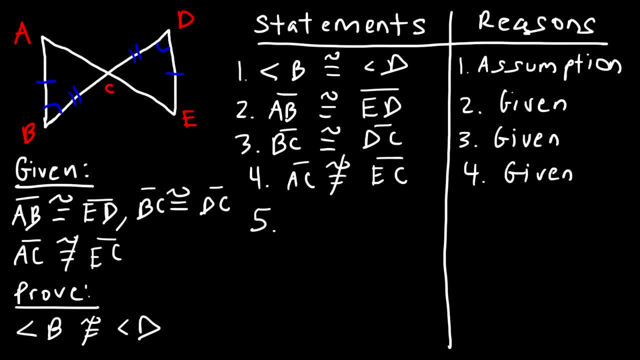 The figure for that. Now, number five, We can prove that the two triangles are congruent Using the side angle Side postulate. So we're going to say that triangle ABC Is congruent To triangle. Let's see. 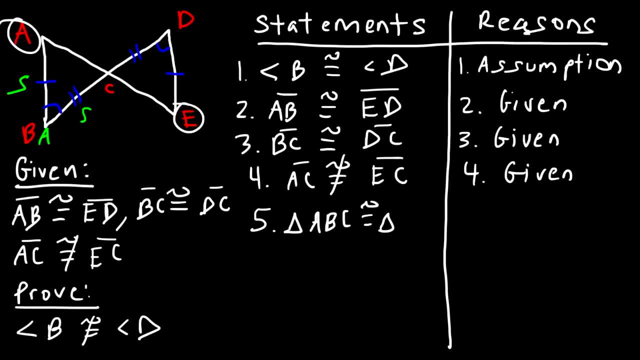 A corresponds to E, So this is going to be triangle EDC. D corresponds to B. As you can see, These two angles are congruent And this is Based on the SAS postulate And This is based on statements. 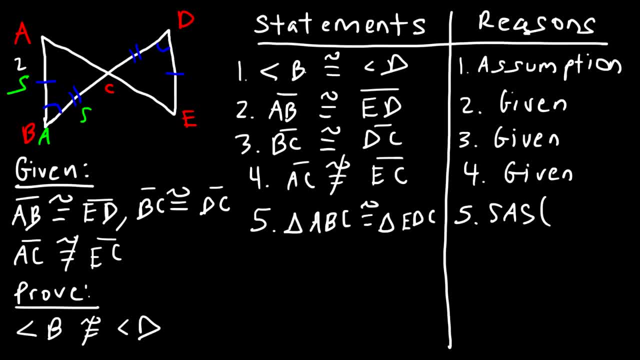 Two, That's with AB. Angle B was based on Statement one And BC was based on Statement three. So this postulate was based on statements Two, one and three. So now number six. Let's focus on 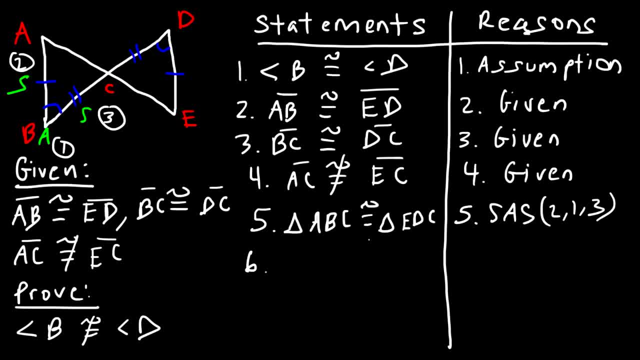 The statement. that's not true. So if the two triangles Are congruent, That means that AC Should be congruent to EC Based on CPCTC. However, We can clearly see that statements four And six contradict each other.